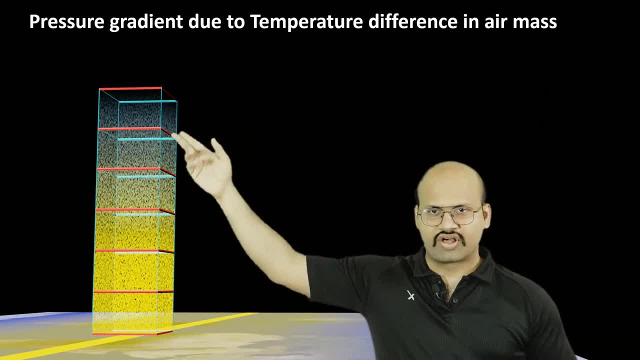 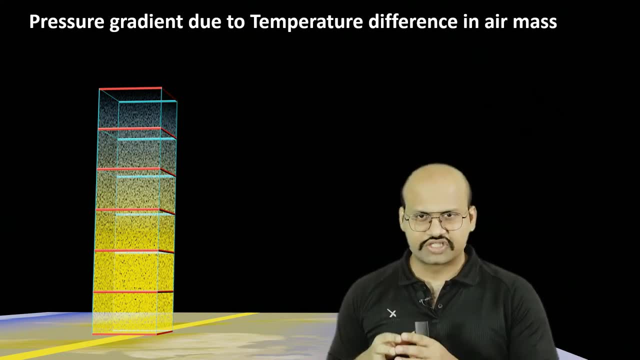 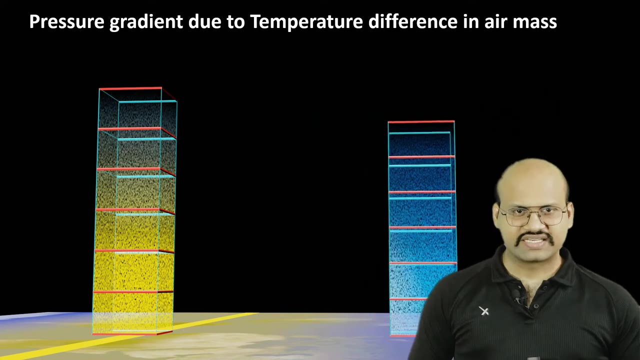 situated at the equator, and this is the air column. The red lines indicate the pressures at different heights. Now, this air column, which is situated at equator, when it moves towards the poles, We can see that the height of this air mass decreases because of the air cooling down. 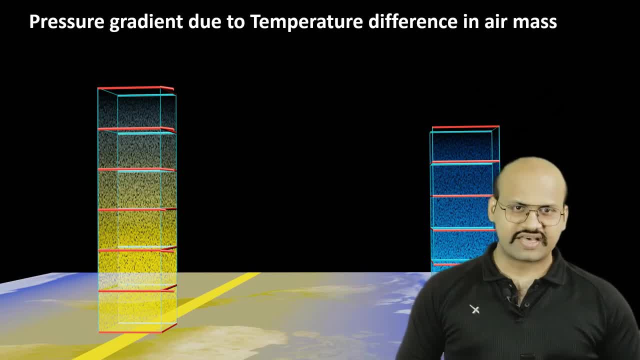 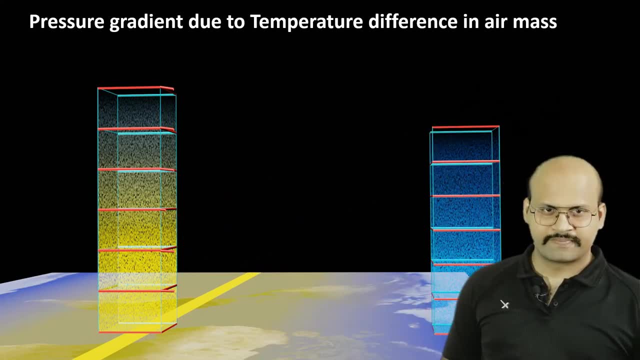 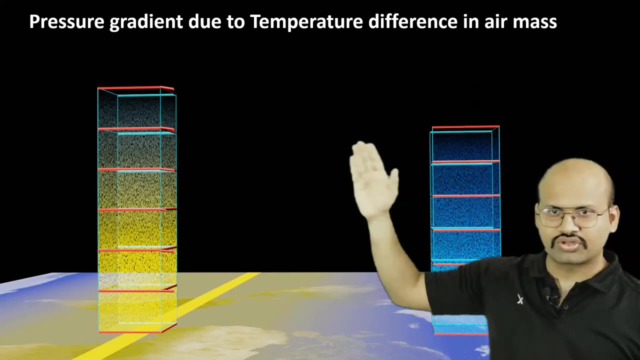 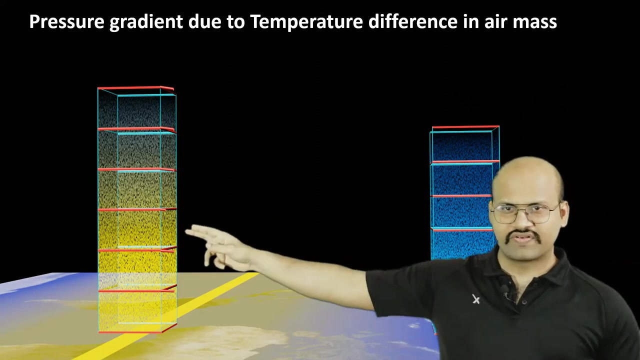 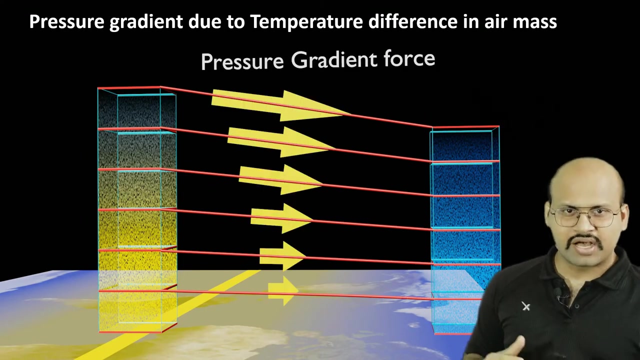 and when it cools down, the density increases And therefore the same amount of air mass which was here. it requires less volume to occupy the air column. Now let's consider the temperature value of our earth. We can see that the air is dissipating. In this case, we can see that it is not dissipating as high And therefore we can see. 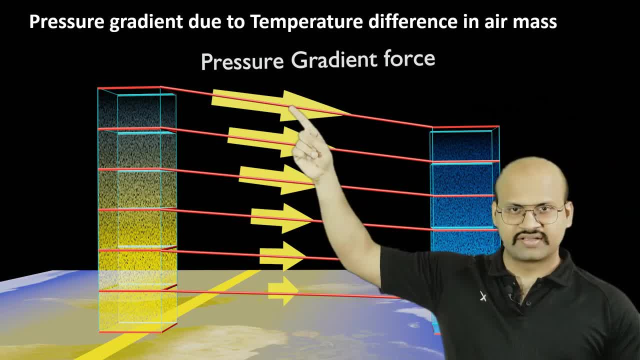 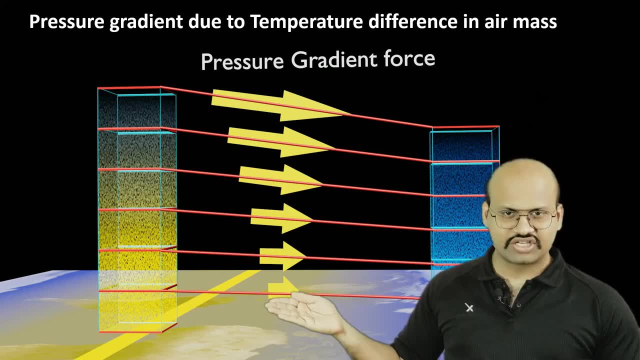 that the height of this bar is smaller, even though the amount of air in both of these columns is similar. We can see that these pressure bars, which we have marked over here, are also located at Lower atmosphere, that is, near the surface. we see that the pressure gradient is not that. 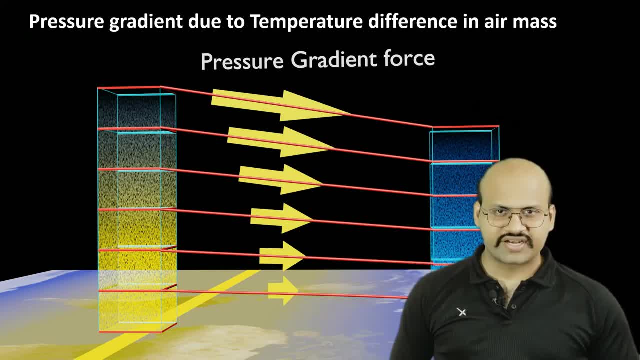 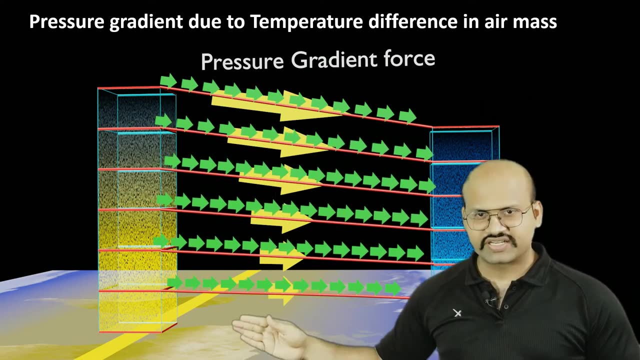 much effective, but in higher atmosphere the pressure gradient is very high. because the difference in pressure is very high in these two columns And due to this higher pressure gradient we see that the winds in the higher atmosphere move at a very high velocity, while the winds at the surface moves at relatively less velocity. 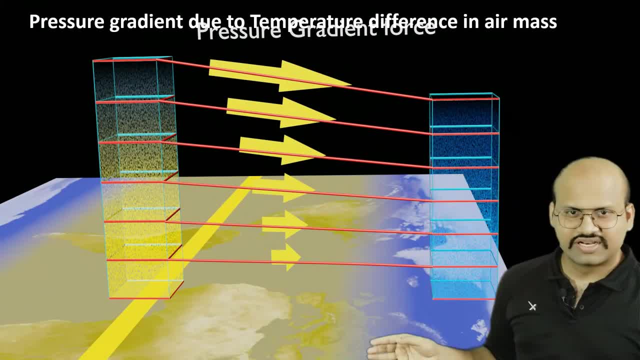 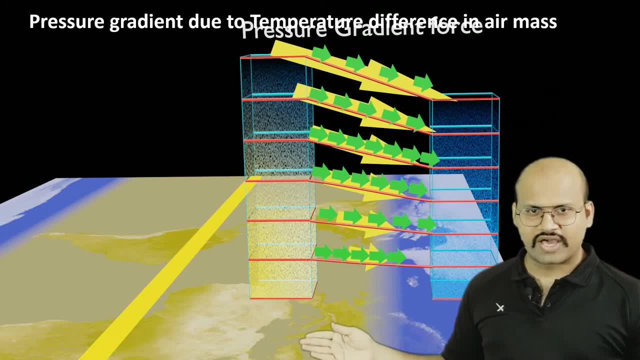 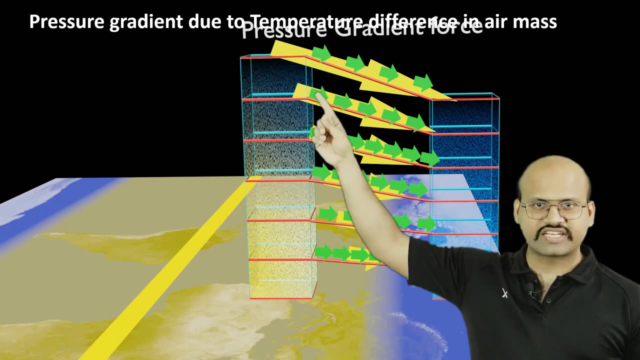 Now, in the higher latitudes, that is, around 60 to 40 degree, we see that there exists a front. We see cold air mass over here and warm air mass over here, and here is a front. So at this front there is a drastic change in temperature, due to which a very large pressure. 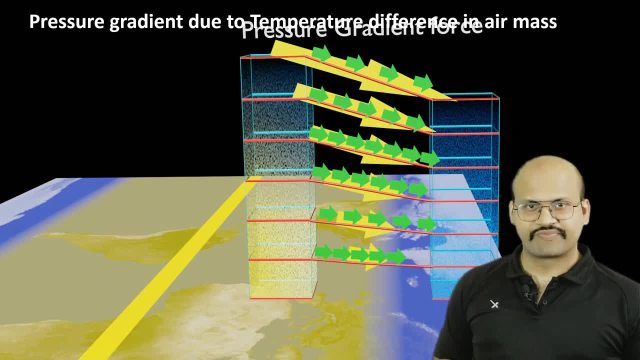 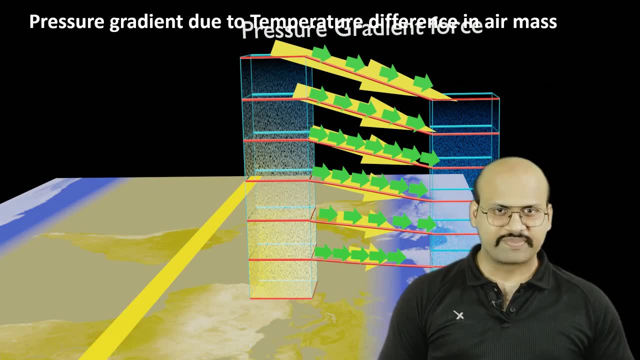 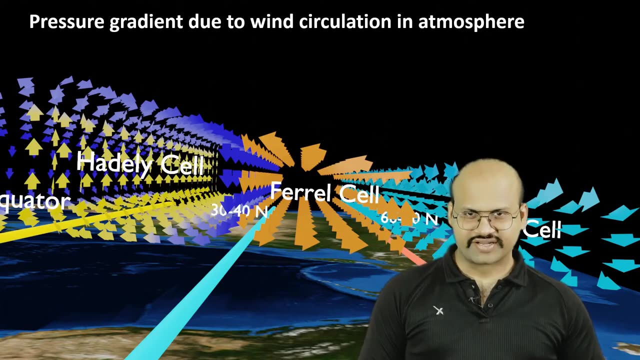 gradient exists here in upper atmosphere, due to which the air moves at a very high velocity. Now remember this high velocity is important because Coriolis force depends on velocity. Now let's see how wind circulation creates pressure gradient. We can see here Hadley cell, Ferrel cell and Polar cell. 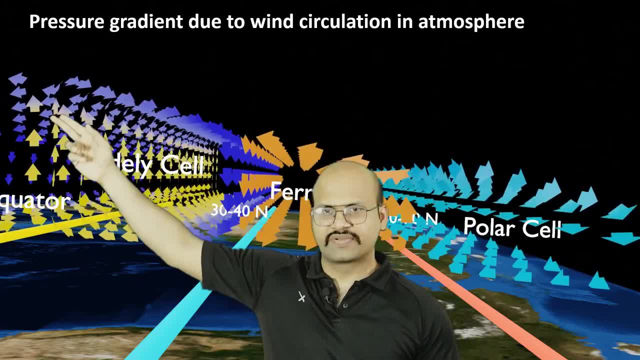 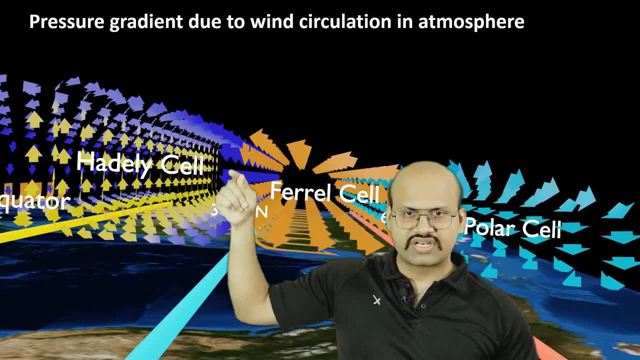 Now, over here in the Hadley cell, the air is rising up. therefore there is accumulation of air over here And this Hadley cell. when it comes over here, the air goes downwards, it descends, therefore there is depletion of air from here. So we see that in a way there is a low pressure region in the upper atmosphere. 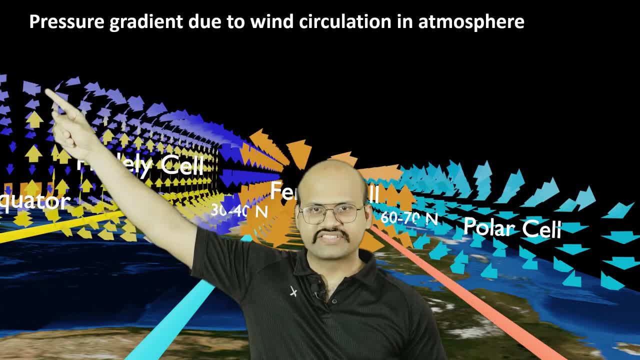 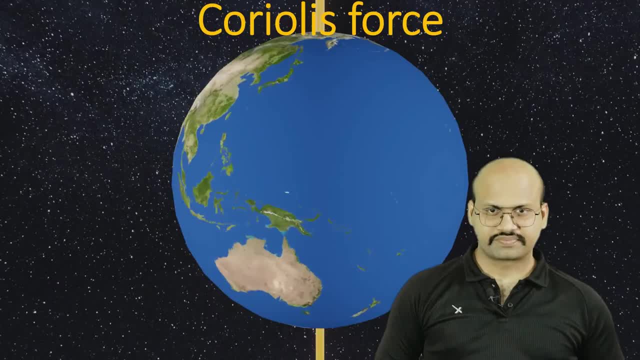 And here there is a high pressure region and due to which there is a pressure gradient. So this is how wind circulation also creates a pressure gradient in the atmosphere. Now let's discuss Coriolis force. We have already discussed Coriolis force in detail in another video. 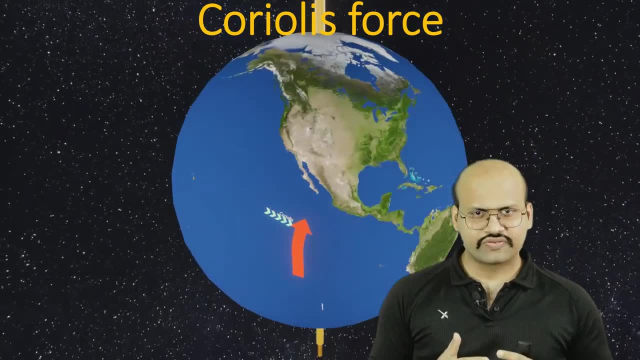 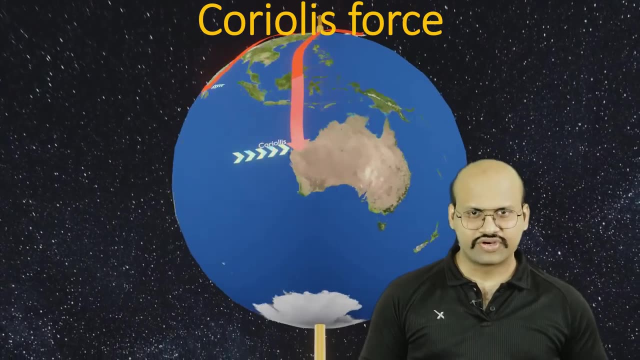 The link for which is available in the description. Coriolis force exerts a deflective force on any fluid. In the northern hemisphere it applies a rightward movement on any fluid, and in the southern hemisphere it will apply a leftward deflection. 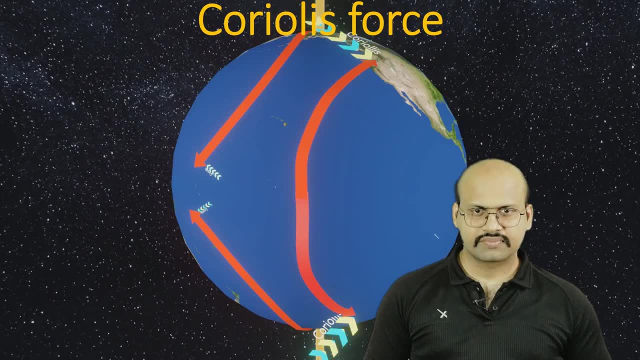 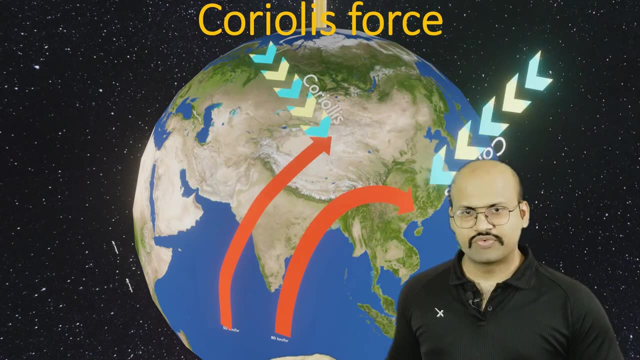 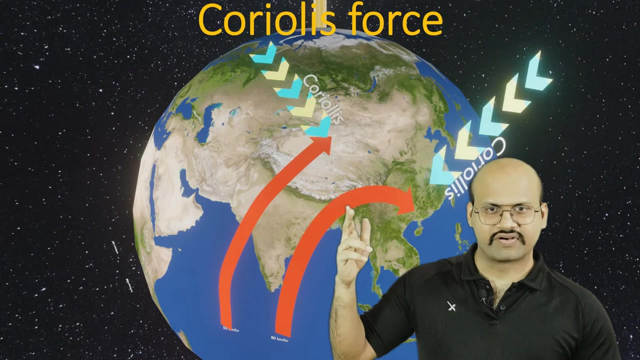 Moreover, the Coriolis force is directly dependent on the velocity of the fluid. If any fluid which is moving fast, then it will experience more deflection. as you can see over here, This wind current is moving at 80 km per hour, while this was moving at 50 km per hour because 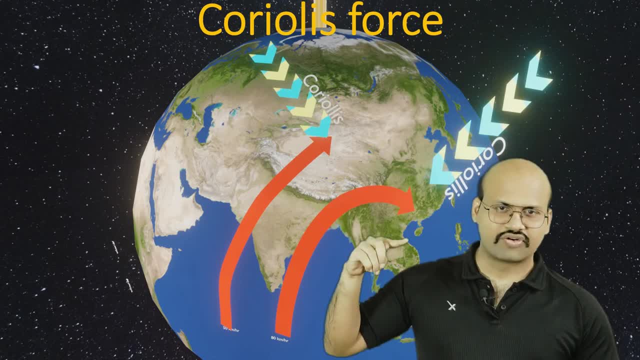 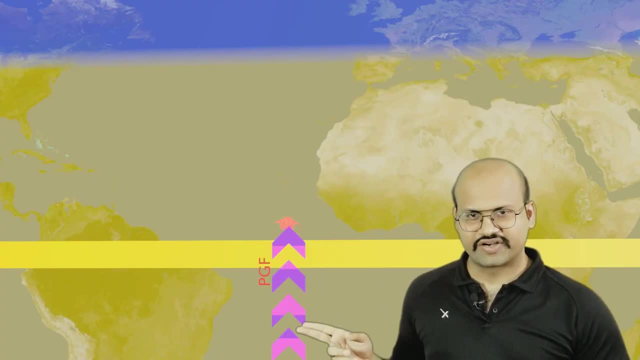 of which this air column got a large amount of deflection. Here we can see an air stream. This air stream is active. This air stream is active by a pressure gradient force. This pressure gradient force tries to move this air stream in the northern direction. 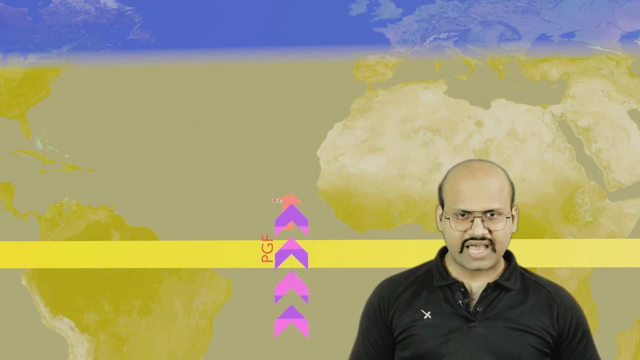 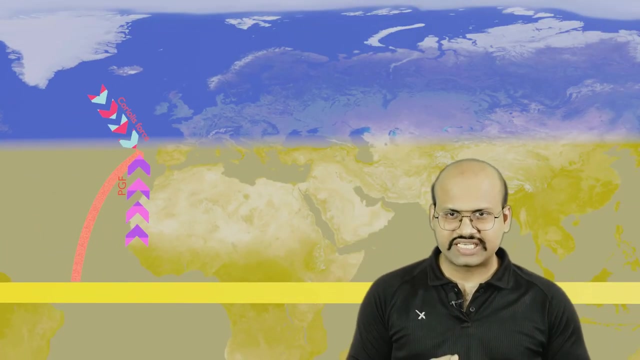 Now, right now, there is no Coriolis force, But as this air stream starts to move northwards, a Coriolis force acts on this air stream. Over time, the Coriolis force increases with the velocity of the air stream, And as this air stream continues to move northwards, its velocity increases and there comes a time. 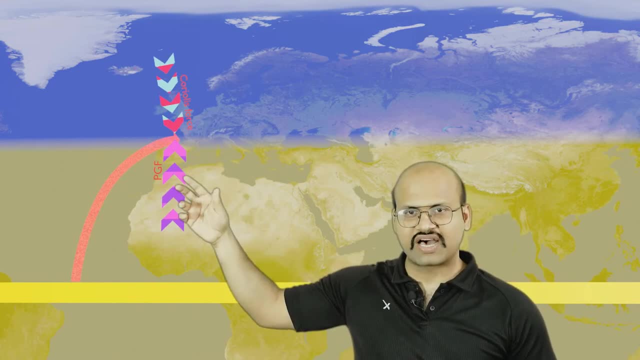 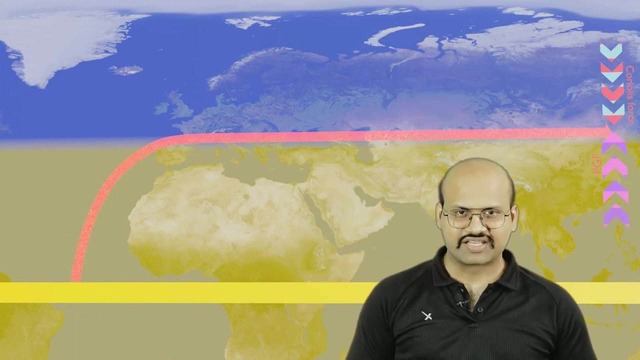 when the Coriolis force and the pressure gradient force are even And in opposite directions, facing each other. It is in the balance of these two forces. we see that the air stream will move parallel to the latitude. It will not be able to go north of this and both of these forces balance each other out. 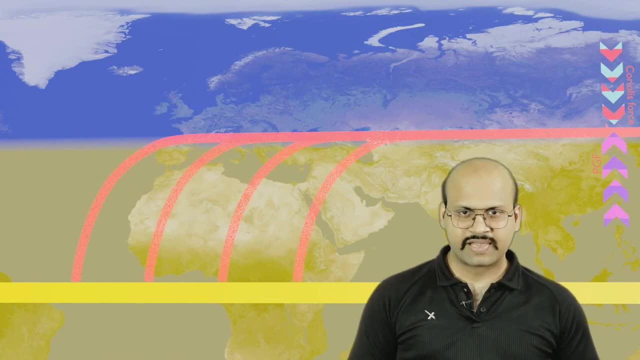 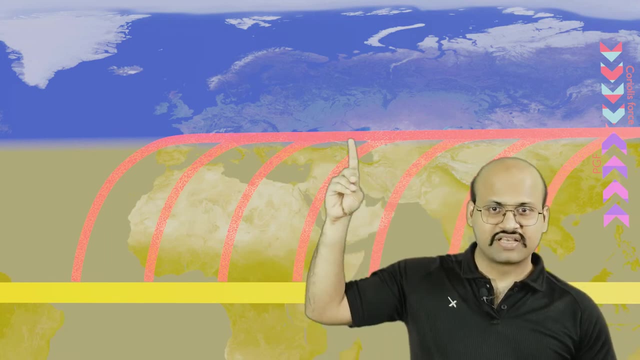 making this air stream to move in a parallel line. This kind of phenomena we can see for several air streams. We can see that there are different air streams and they all move in this direction. Therefore, the accumulation of these air streams over here It leads to a different air stream. Therefore, the accumulation of these air streams over here It leads to formation of jet streams. These jet streams are situated 10 to 16 km higher in the atmosphere and that is why they move with such greater velocity. These jet streams are around 200 to 300 km wide and they are formed of different layers. 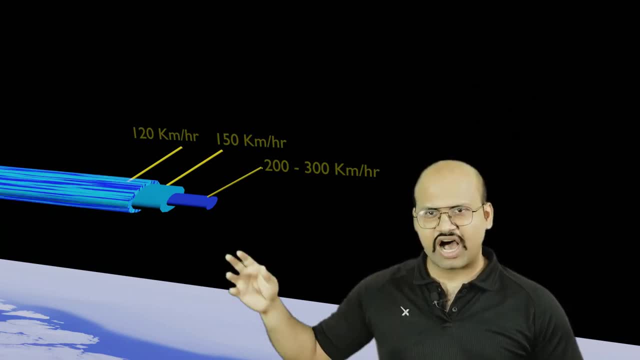 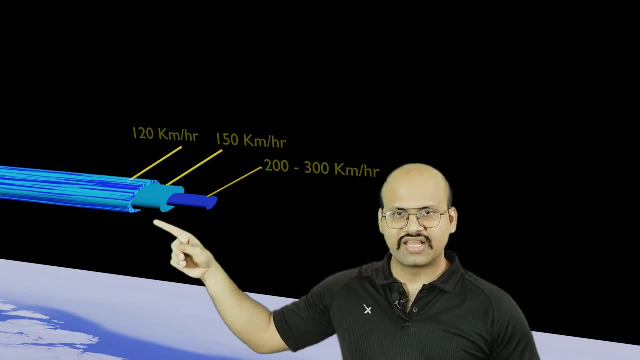 and each layer has different velocity. We can see that the outermost layer is the slowest. It has a velocity of around 120 km per hour. The outer layer is the slowest, The middle layer has velocity of around 150 km per hour and the inner core has the highest.